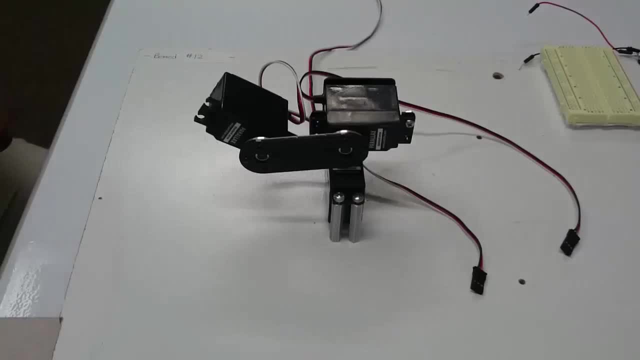 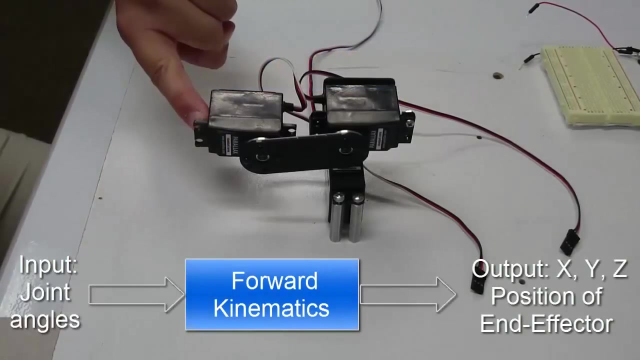 The angle of each of these joints. Today, we're starting to work on a robotics problem called forward kinematics. The problem of forward kinematics is: how can I find the location in space of the end effector, given the angles of each of the individual joints? 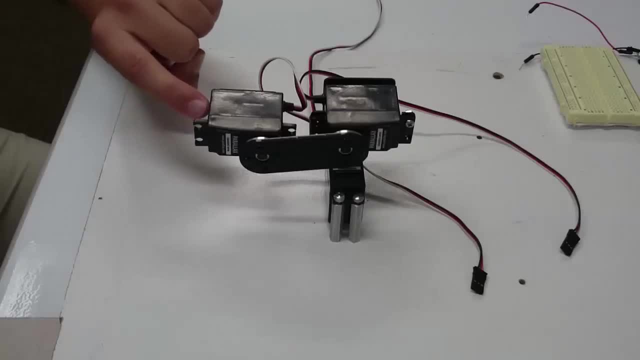 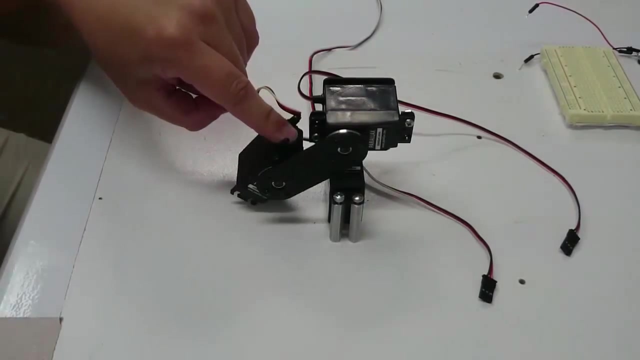 If I can do that, if I can find the location of the end effector, given the angles of each of the individual joints, I can avoid sending a command to each of my servos that will place the end effector in a position I don't want, such as colliding with the table. 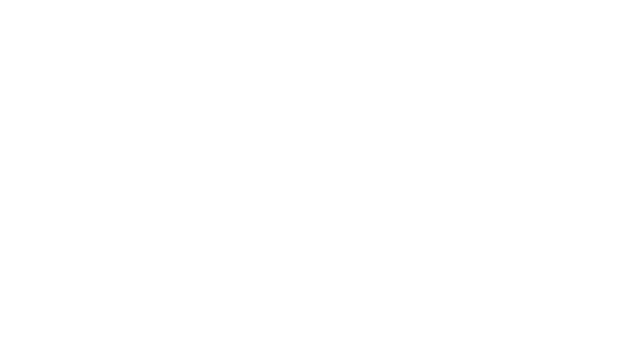 The key to finding the location of the end effector, given the angles of the joints, is a special kind of a matrix called the homogeneous transformation matrix. The homogeneous transformation matrix is a kind of a matrix that has four rows and it has four columns. 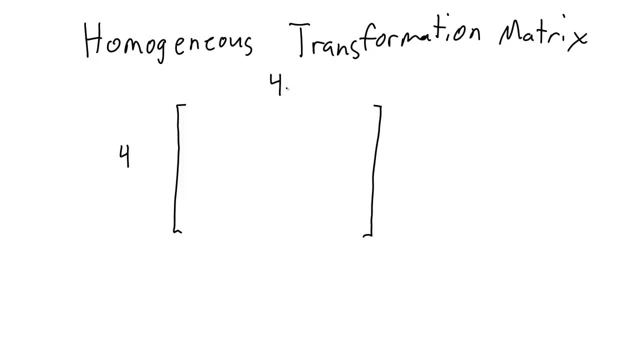 and this matrix encodes two important things about our manipulator. This area right here, which is three by three, tells us the rotation of one frame in our manipulator relative to another frame. This vector here, which has three rows and one column, 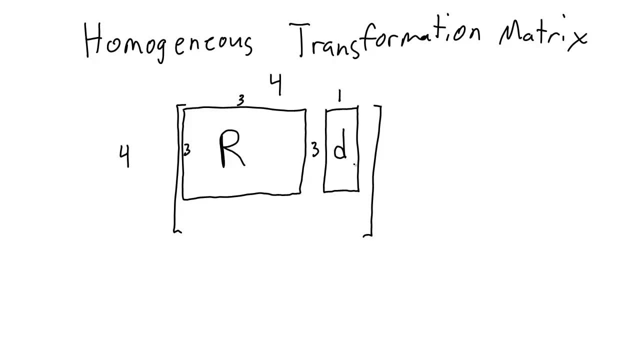 it tells us the displacement of one frame relative to another frame. The rest of the homogeneous transformation matrix is easy. it's just three zeros and a one which we fill in to make the matrix square. so four by four, Once we figure out the rotation matrix,